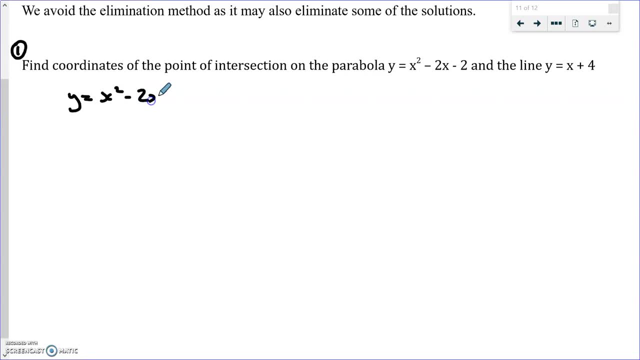 x squared minus 2x minus 2 and y equals x plus 4.. So you can already see, both of the equations are equal to y. So we can make the two equations equal to each other. So I'm going to substitute equation 1 into equation 2.. So x plus 4. 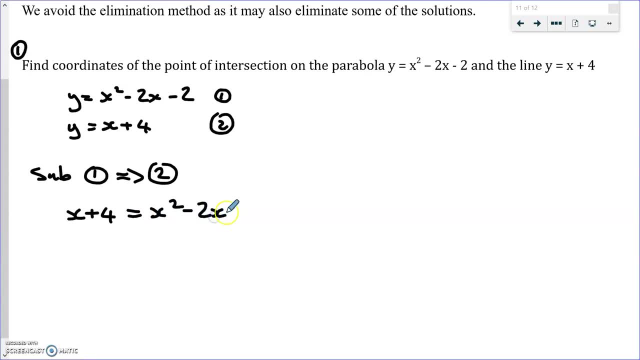 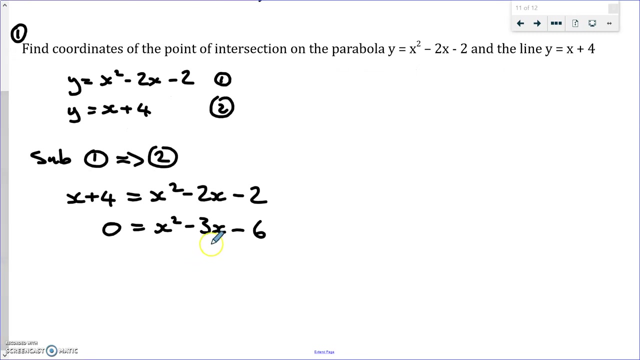 equals x squared minus 2x minus 2.. Let's take everything over to subtract x, subtract 4.. So x squared minus 3x minus 6.. Okay, so to solve this I'm going to use the quadratic formula. So you might remember to use the quadratic formula. I'm going to say a equals 1, b. 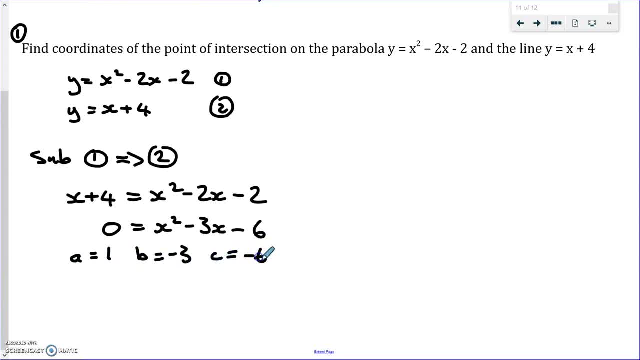 equals minus 3, c equals minus 6, and I'm saying x equals minus b, plus or minus, plus or minus root of b, squared minus 4ac, all over 2a. Okay, so I'm going to keep going, Just a bit more. 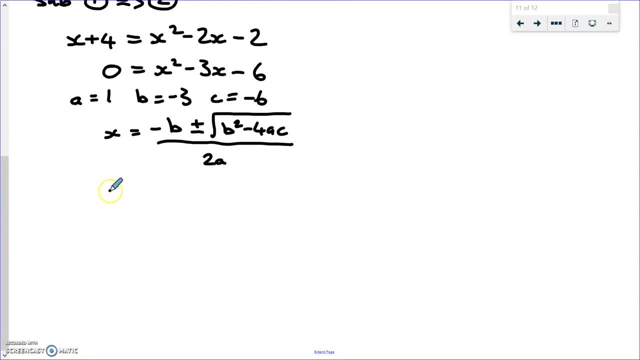 space here. Okay, so x equals minus minus 3, plus or minus 3 squared minus 4 times 1 times minus 6.. And I want the square root of all of that, and all of that over 2 times 1.. 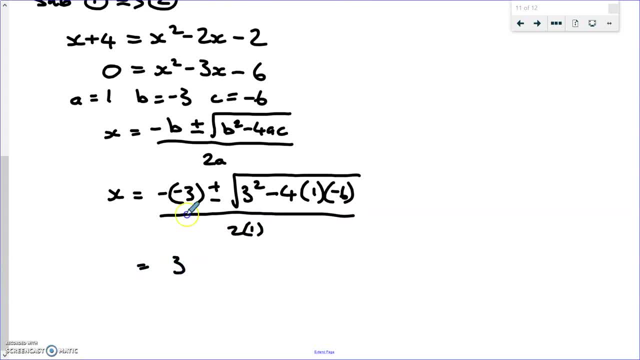 And then I'm going to keep going. So it gives me 3 minus and minus plus or minus 9 minus 4 times 3 times 4, 6 is 24, plus 24, minus times a minus all the way to about 2.. 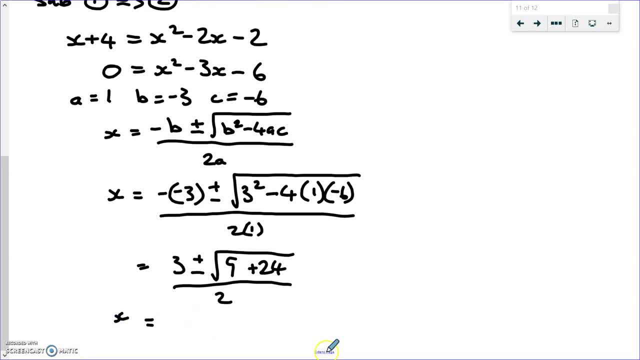 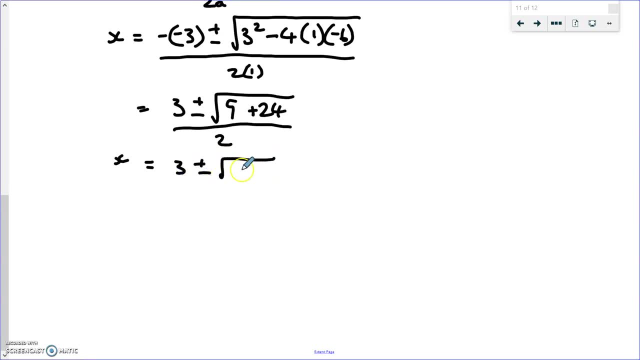 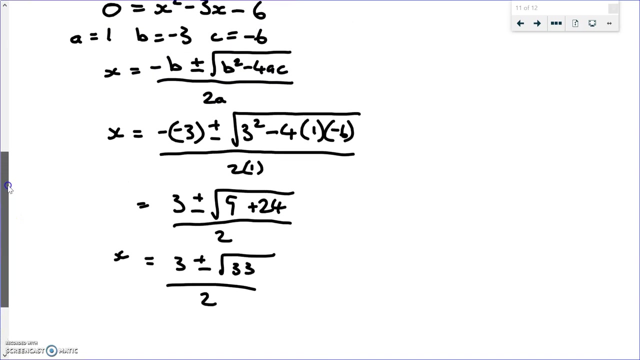 So I end up with: x equals the square root of 3 plus or minus the square root of 33 over 2.. Now I'm going to leave it as an exact value. Now go back up here. Let's find this equation: y equals x plus 4.. 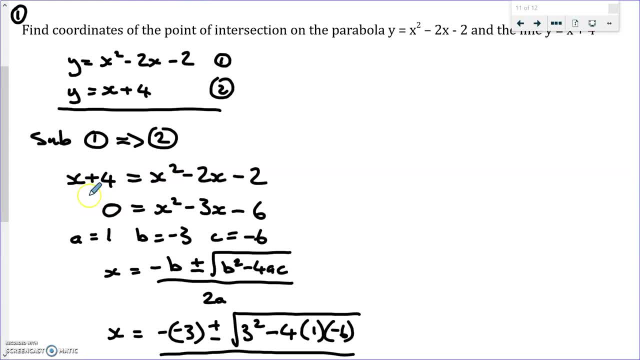 I'm going to just substitute that. I'll just cross it out a little bit. I can't say that and I'll cut that into. I'm going to substitute that in. So let's do this up here. Let's substitute in: x equals 3 plus or minus planet. 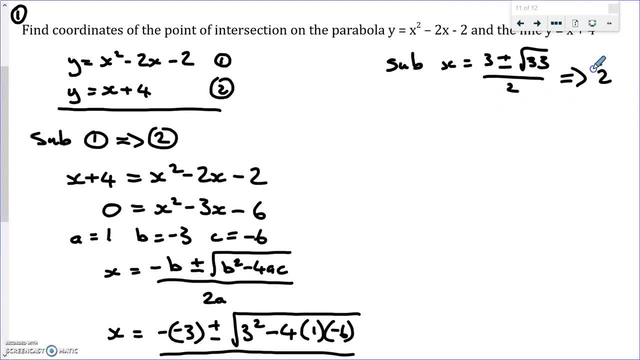 square root of 33 over 2 into equation 2. And so y equals 3 plus or minus square root of 33. from Sis到 restore Cr vardır 33ius sistema, demonstrate 2 plus 4.. Let's put it all on this common denominator Plus 8 for the 2.. 3 plus 8 is 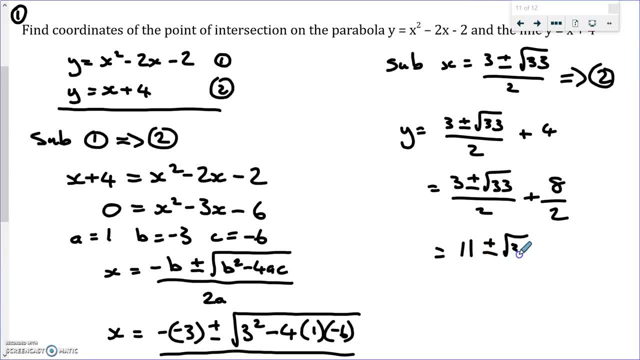 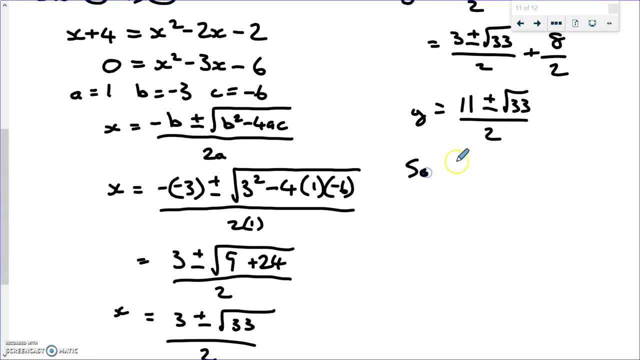 11 plus or minus root, 33 on 2.. Now, what do we have? We've got 2 x's and we've got 2 y's and we need to put them together. so our coordinates become 3 plus root, 33 over 2 and 11 plus root. 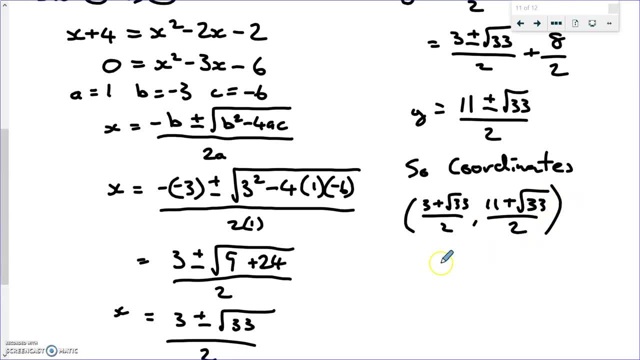 33 over 2.. You can make some decimals, but we try to keep them as exact values as we can, And the other coordinate would be 3 minus root 33 over 2 and 11 minus root 33 over 2.. And so there our two. this particular set of equations intersect at two points. 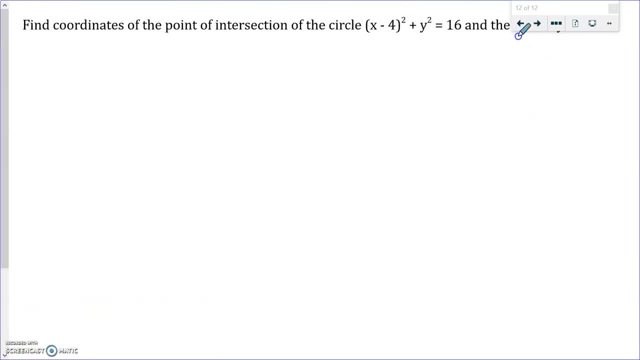 Okay, so that's it, Thank you. Thank you, Let's do one more. So, number 2, find the coordinates of the point of intersection, or points of intersection on the circle x minus 4, all squared plus y squared, equals 16, and the line: 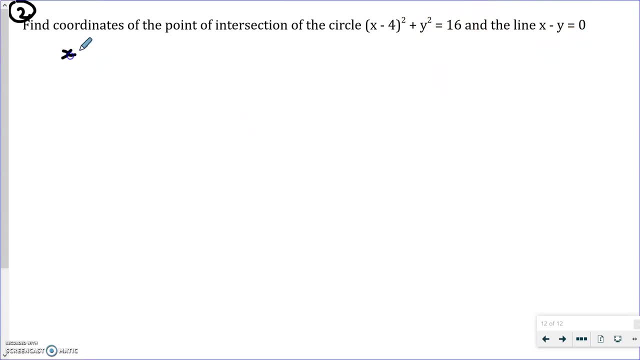 Again, we're going with our equation. you know, x take 4 all squared plus y squared equals 16.. That can become equation 1.. Okay, So x minus y equals 0.. That can become equation 2.. I'm going to rearrange equation 2 to become y equals to x. 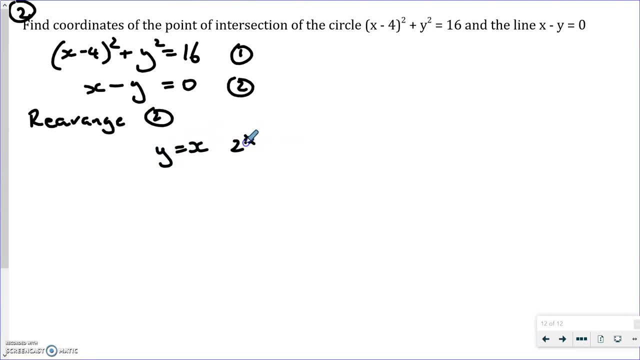 So that's my 2 star. I just rearranged it And I'm going to substitute. Come on going to substitute. so substitute two star into equation one. so equation one: x minus four, all squared plus x. I'm substituting: x equals y, so instead of y, 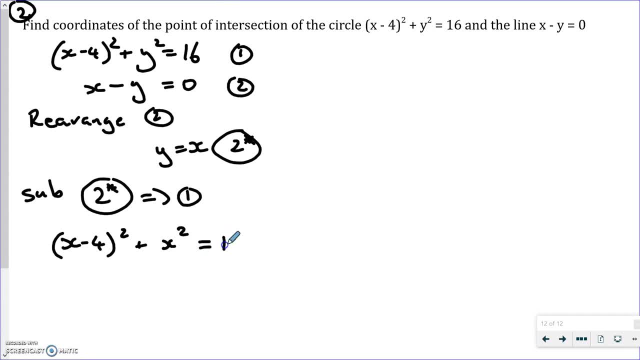 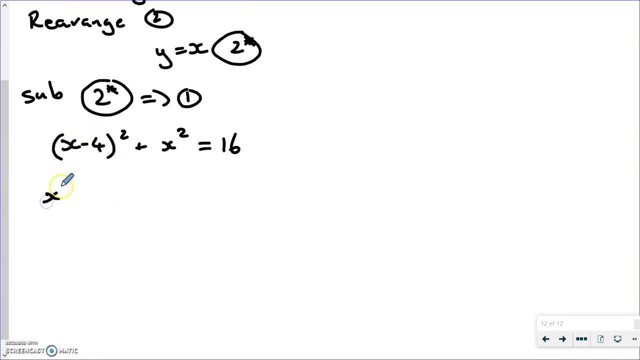 I'm putting x equals 16. make a little bit of algebra. now let's expand this bracket: x squared minus 2 times 4 times X, so that's 8x plus 16 minus 4 times 4 plus x squared 16 plus 16, on both sides, minus 16. cancel out. so. 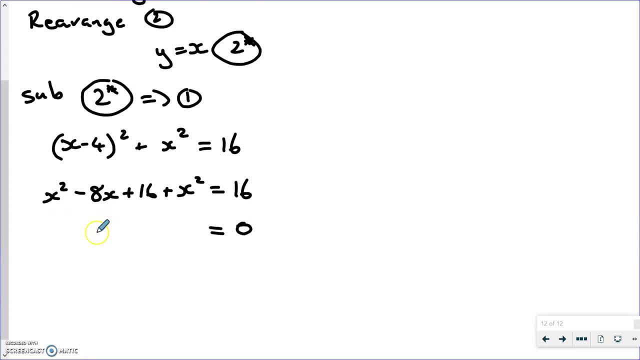 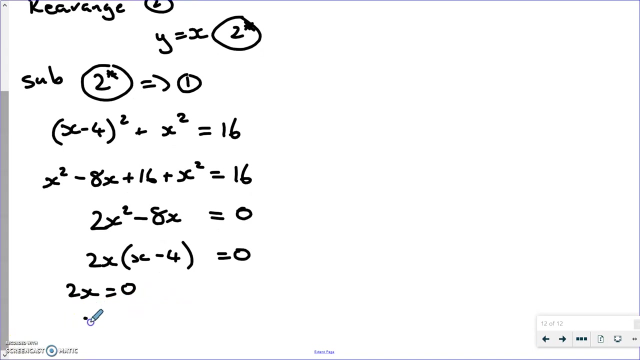 it's, we're gonna end up with 0. on this side we're gonna have 2x squared minus 8x. take 2x out as a common factor. x minus 4 equals 0. so 2x equals 0 gives me x.